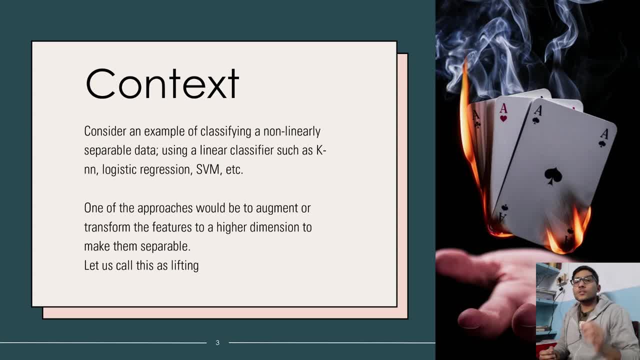 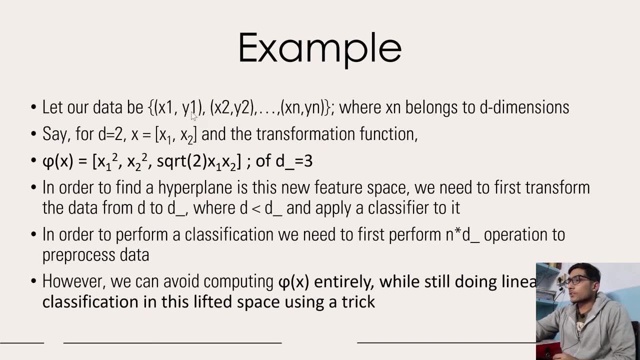 separable. Now this augmentation technique. let us call this lifting. for a while, It may be referred to as something else. We are not aware of it. Let us call this as lifting. Now the example. Let our data be referred to as vectors: x1, y1, x2, y2, xn, yn. So. 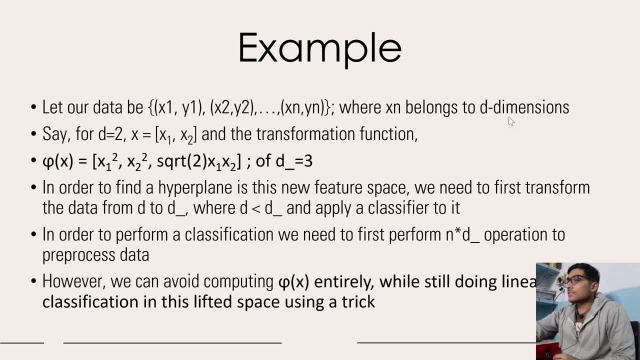 there are n data points And this xn belongs to d-dimension, So each of these are d-dimensional vectors. Now say for d equal to 2, as for example here. So we will have: x is equal to x1, x2,. 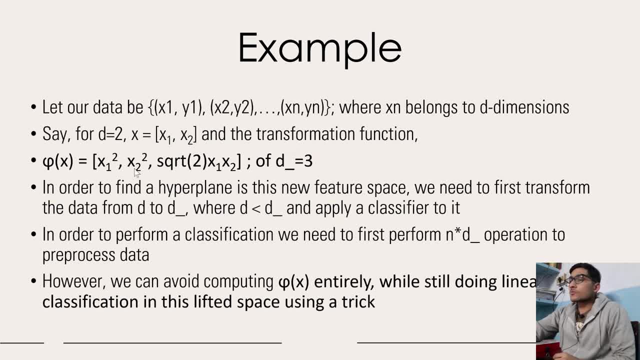 and the transformation function is defined as x1 square, x2 square, square root of 2, x1, x2.. Just understand what I am trying to say. Just do not try to make a logical conclusion of it yet. Just understand the example that we are laying forward. So this is a transformation function. 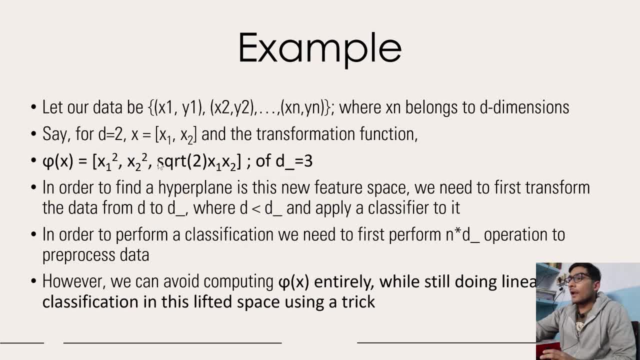 which will apply to our vector. in order to get this- And the dimensionality of this transformed vector is now 3, because we have 3 parts to it- Earlier d was 2.. Now d dash is 3.. Now, in order to find a hyperplane in this new feature space, we transform our original vector x. 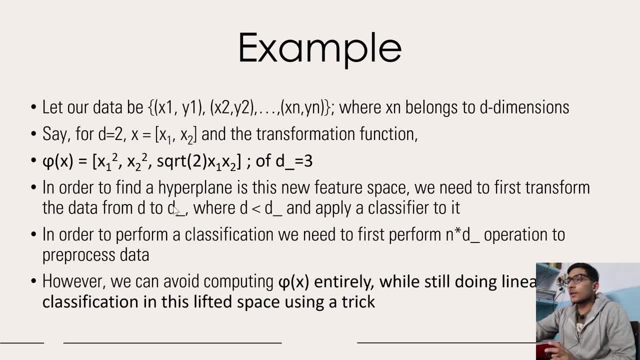 to this new feature vector, phi x, And this phi x is such that d dash is greater than d. OK, Now, in this new feature space, in this higher dimensional feature space, we can apply the linear classifier and classify our data set. OK, Now everything looks good. 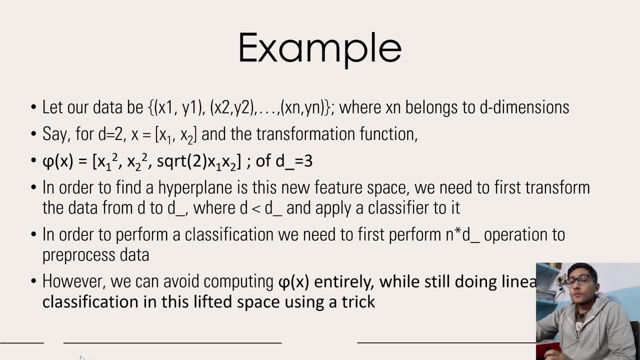 142, 00 조�. 246, 004, 249, 008, 4099, 4099, 007. What if we could avoid computing phi x entirely while still doing linear classification in this lifted space using a strict? Now why we will call this as a trick, because it is rather a hack. 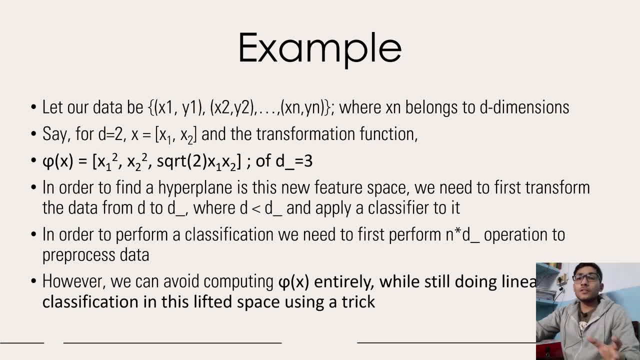 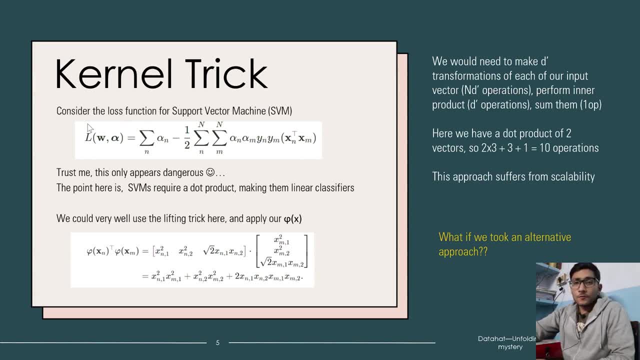 okay, it is a hack. it is not a complete method in itself. Okay, now, coming to the kernel trick. You must have heard of SVM. if not understand that, SVM is a linear machine learning classifier. We shall discuss about SVM in detail in a separate video. but just understand, it is a 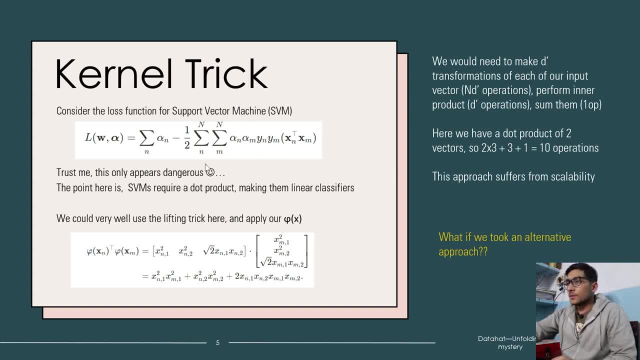 machine learning classifier and the loss function of this SVM support vector machine is given as this. Okay, just do not try to understand each of the different variables given here. it might appear dangerous as well, but it is not. it just uses a lagrange multiplier and the different mathematical 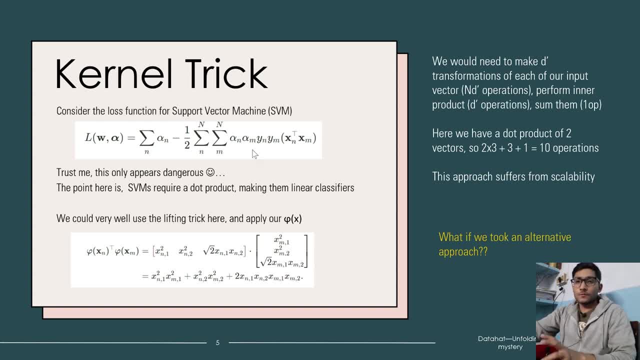 concepts and it is a dual form of the original loss function, which is the hinge loss. Okay, now just take it for my word that this is the loss function for SVM. Now you see, this loss function contains a dot product, dot product between xn and xm, So dot product between the two inputs, Inputs, basically the 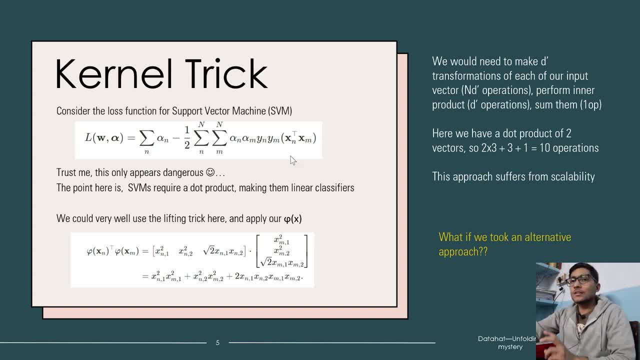 data points. So, since it contains a dot product, it is a linear classifier. Okay, understand this. Now our point here is SVM is: it requires a dot product. therefore they are linear classifiers. We could very well use the lifting trick here and apply our transformation Now. we could very well. 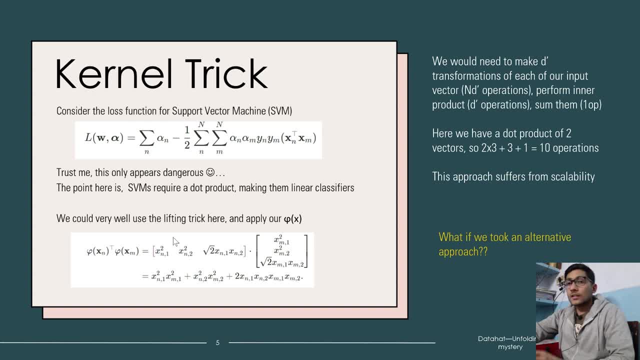 apply our transformation Now. we could very well apply our transformation Now. we could very well apply our transformation in this space using our lifting technique, which we refer to as lifting, and convert it into this space. Now what happens is the number of operations that we require for. 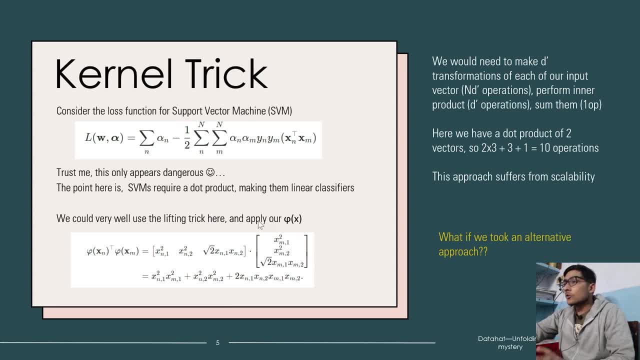 this process is: first we have to make the feature transformation. So we would require d dash operations because d dash would be the new dimensionality, So d dash operations. So understand now, if we have n data points, it would be n d dash. Then we perform an inner product on those d dash. 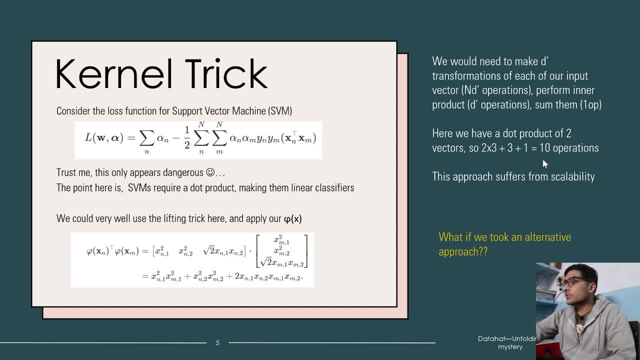 Okay, this is the inner product, So we would have an inner product on those d dash. Okay, this is the inner product product. we have 3 cross 3, so 3 operations. and then sum them up. so just for this, this example, if you consider we would have 2 into 3, because we have 2 vectors, so 2 into 3, 6 operations plus 3. 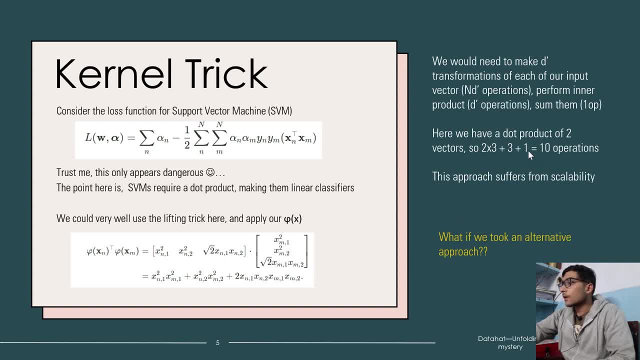 dot: 3 summation operations- okay and 1 sorry. 3 inner product operations. we had 6 transformation operations, 3 inner product operations and 1 summation operation, which equals 10 operations for just this one particular one. for this specific data points: 2 data points- okay, so we'll. 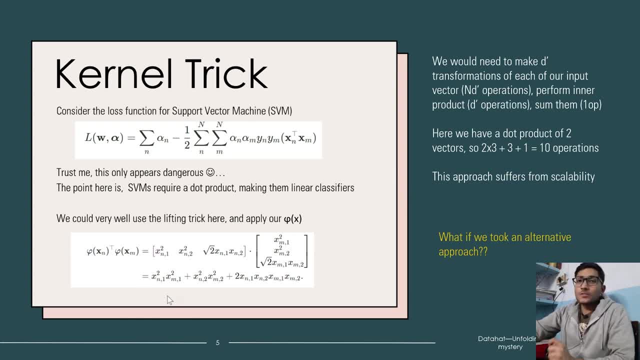 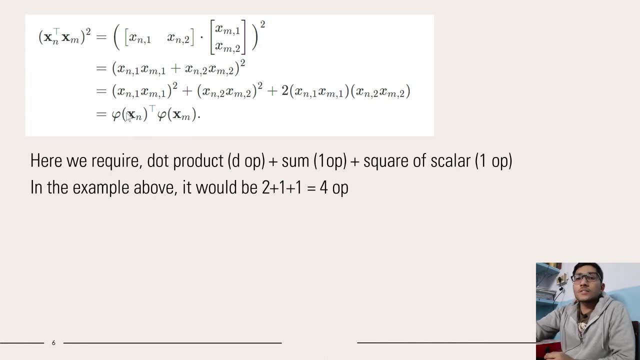 have 10 operations. now the problem with this approach is scalability. what if you want to scale it up? okay, there would be very challenging in terms of the computational resource that you require. what we take an alternative approach. now, what is an alternative approach? so the alternative approach is instead of converting or instead of using phi x transformation on our feature. 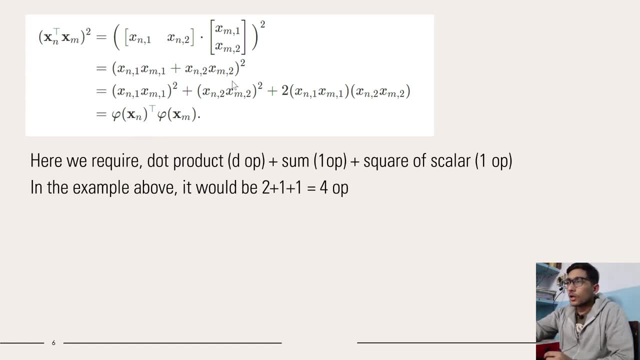 space. what if we first take the dot product, sum them up and then square it up? basically, square is just a function. here the function could vary depending on the kernel that we use. now you understand what is the kernel. the kernel is basically the operation which would be applied. 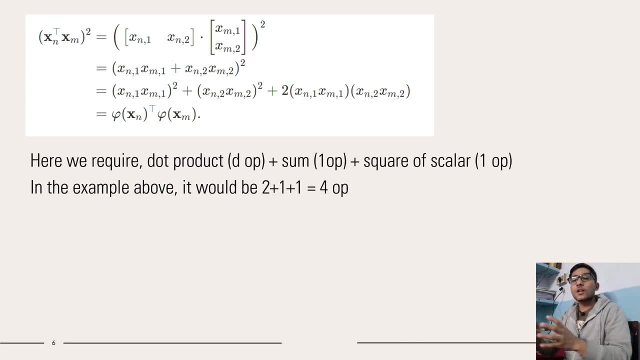 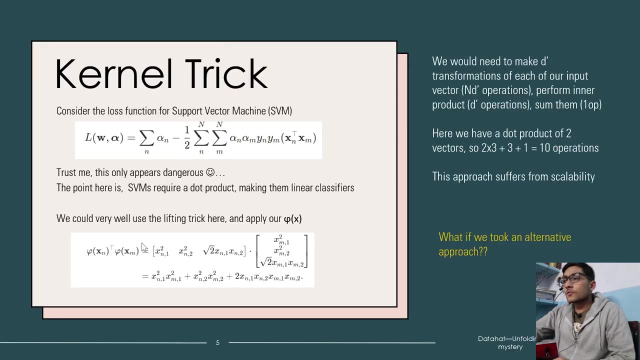 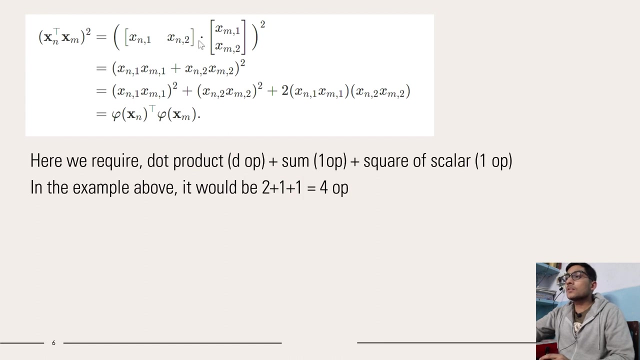 to your dot product or the inner product, such that it transforms your feature space without actually transforming your data points. okay, you see, from this example, when we square this up, you are getting the exact same result as you got using this transformation first. so you first transform them, then you took the dot product. whatever result you got, you're getting the same result when you 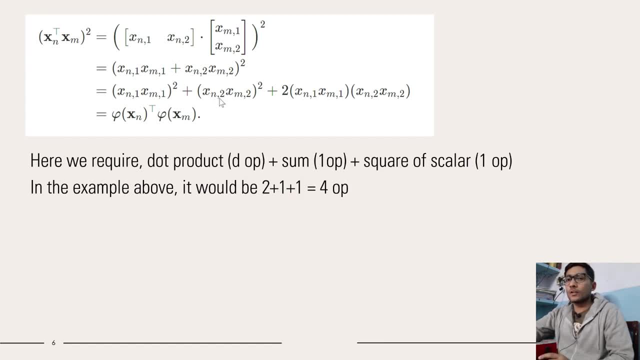 first take the dot product, do the summation and then square it up. now the number of operations that we require in this process is: we require d operations for the dot product? okay, d dimensional d operations, because we don't have any transformation. so no, zero on that. 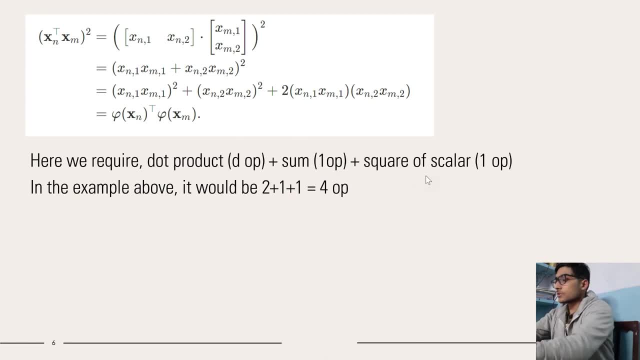 one summation and then one square of scalar, so total four operations. so now we see here that it requires only four operations as compared to 10 operations in case of the lifting trick. that is what makes kernel tricks so powerful. that is why they are extensively used in svm for classifying non-linearly separable data set using linear classifier. that is svm now. 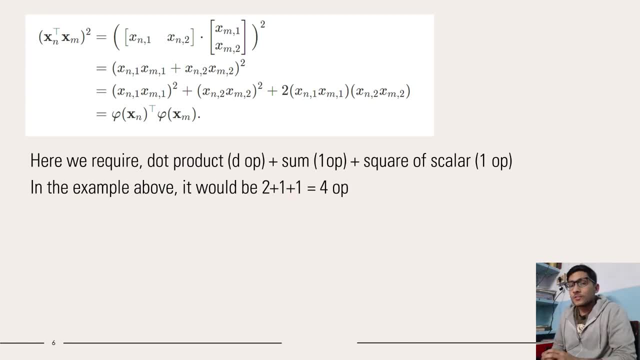 that you are convinced with the power of kernel trick and why that is called as a trick. I would again request you: if you haven't subscribed to the channel yet, make sure to subscribe. hit the bell icon, because we are going to bring a lot more surprises in the coming days, in the coming weeks. 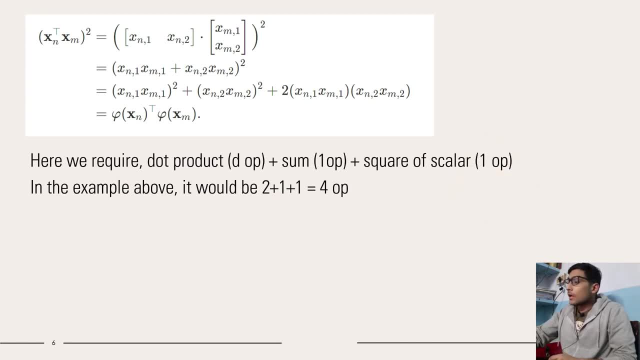 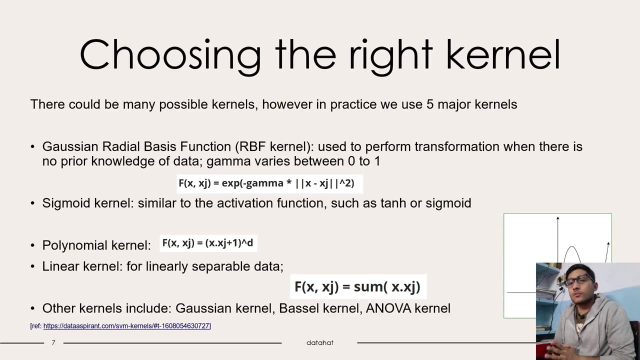 in the coming months and the whole year. so now, next, we'll move on to how do we decide which kernel to choose. okay, very well, I convinced you that you should use a kernel trick, but again, kernel is also a method, whether you should square it up, whether you should a cubit, whether you should take 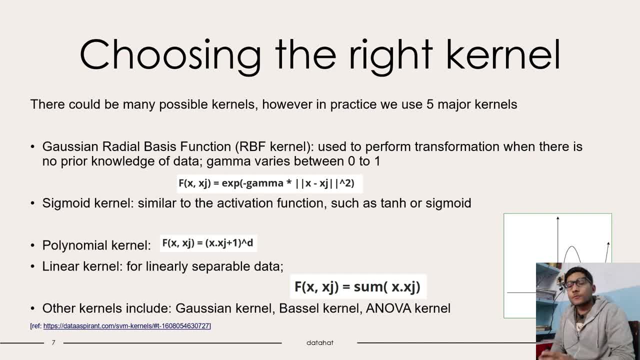 the square root it should bean an odd: okay fine, that you did good and it is of particular importance, should decide it. So now, the burden of this has already been taken care of by data scientists over the years, and they have shortlisted certain kernels which perform incredibly well across. 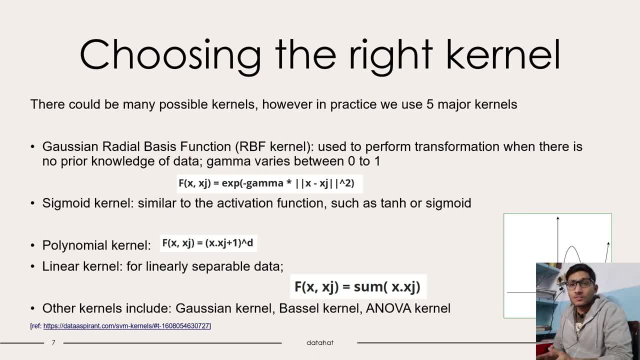 situations, across different situations, across different types of data sets, and here we have a list of some of them. So some of the primarily kernels- major kernels- that are used are the Gaussian radial basis function. This is used whenever you have no idea of what the data set. 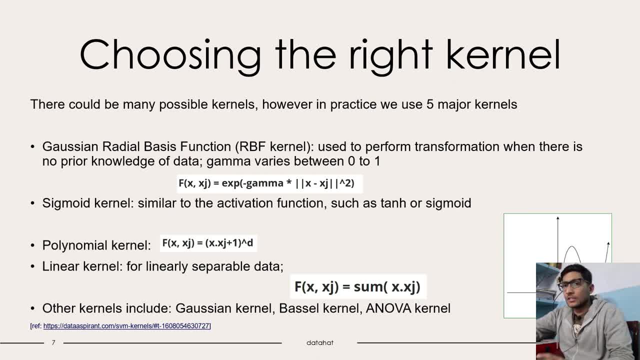 looks like what the data set is about. So you apply a Gaussian radial basis function. However, this is also a complex form, So we first approach it with the simplest of form, that is, a linear kernel, then probably try a polynomial kernel or a sigmoid based kernel and then go for the 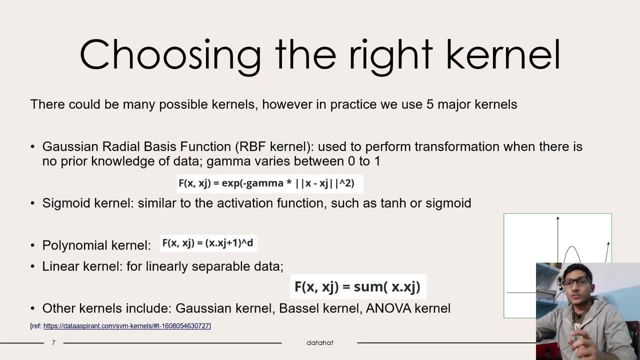 Gaussian kernel. This comes under the process of cross validation. You evaluate your model by using different kernels and see which works best, But you do not have to go in an infinite space to search For your appropriate kernel. you just have to select among these four or five of them. Now you 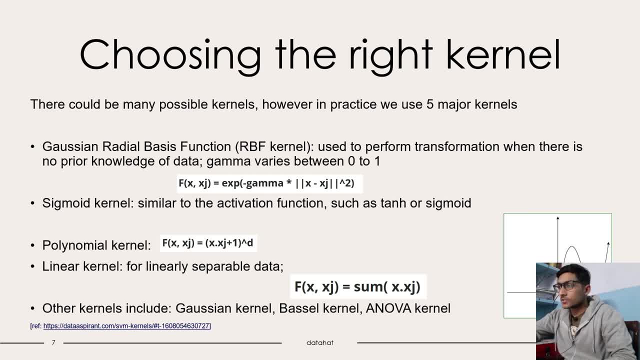 see from here that Gaussian radial basis kernel is a kind of a Gaussian function. Sigmoid kernel is basically similar to the activation function. sigmoid tanh, relu, those things. Polynomial kernel is just the square cube, the different d dimensions, as you can see from the image as well. 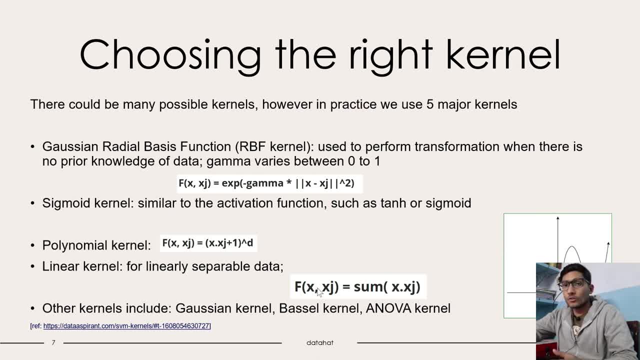 Linear kernel is nothing, just a linear operation on the original dot product. Some other kernels also include a linear kernel. So this is a linear kernel. So this is a linear kernel. So this is a linear kernel. This is a linear kernel. This is a linear kernel. We can also include Gaussian. 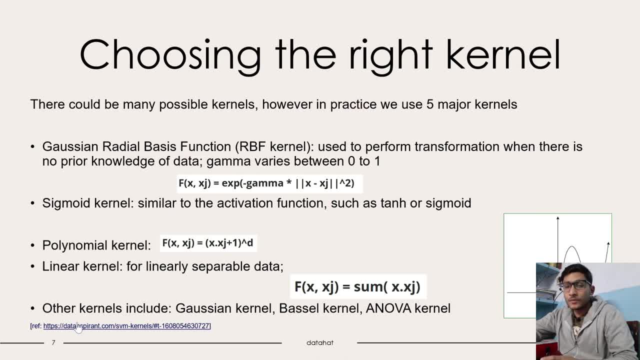 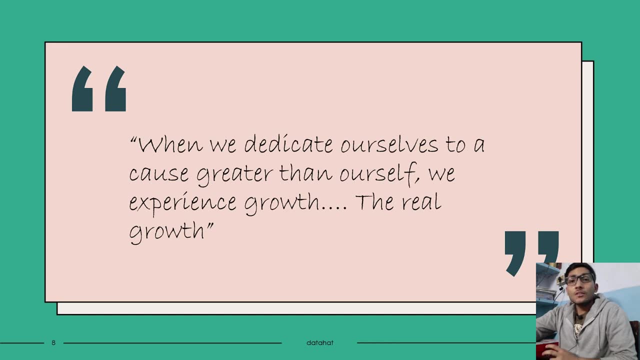 kernel Basel kernel Annover kernel. If you want to learn about these, I have attached the link here on the description. you can go in the description and read them out Now again, as we do in all our videos. here is a small thought for our viewers that when we dedicate 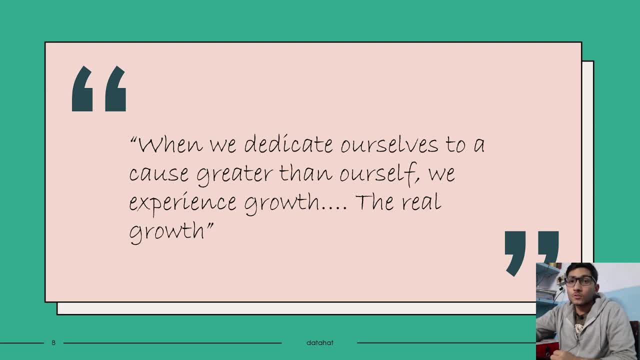 ourselves to a cause greater than ourselves, we experience growth. We experience real growth, And you have to trust me on that. you are going to experience real growth when you dedicate yourself to a cause which is greater than yourself. that cause could be anything that could depend on your dreams, your aspirations, but 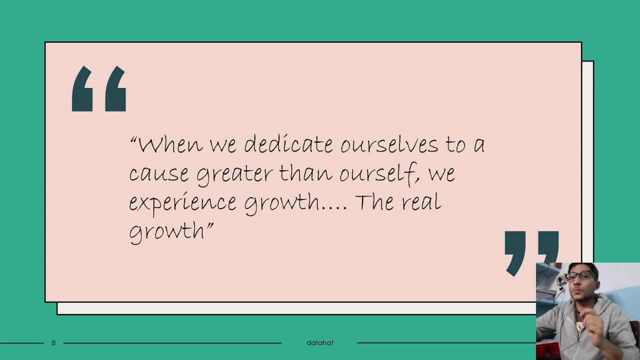 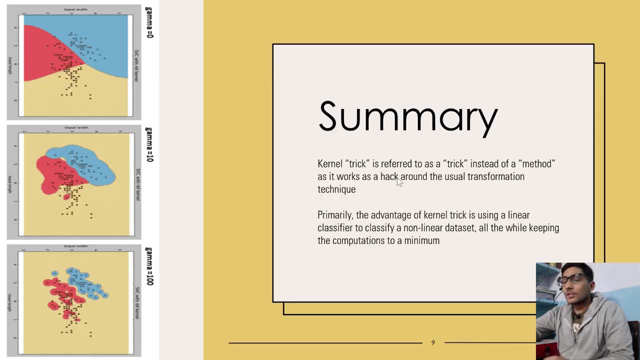 remember to have a cause which is greater than yourself. it will take time, but we'll soon have it. now, coming to the summary of it. we understood what kernel trick and why kernel trick is referred to as a trick and not as a method. what is the primary advantage of kernel trick and how does it classify?